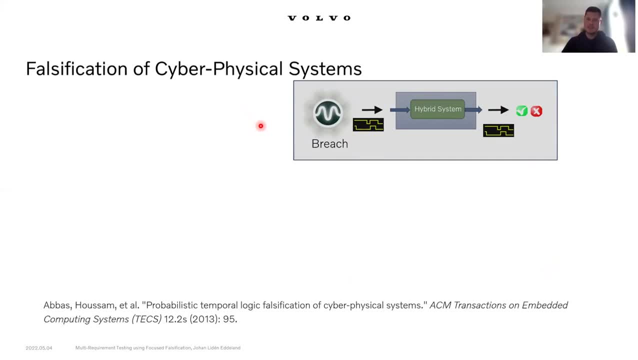 which is a way to automatically generate tests for hybrid systems under test. So what we have is a toolbox in MATLAB called Breach, which we use to generate curves, Which are the inputs to the hybrid system that we simulate. in our case, After we simulate, we get the output from the system. 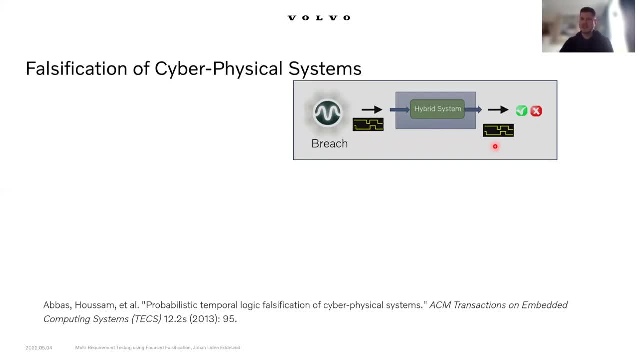 so then, with having requirement or specification in signal temporal logic, we can monitor these outputs and check whether the requirement is fulfilled or not. A more detailed schematic of the falsification procedure, as it is usually used in academic papers, is shown here. So what we assume is that the input to the system is parameterized in some way. 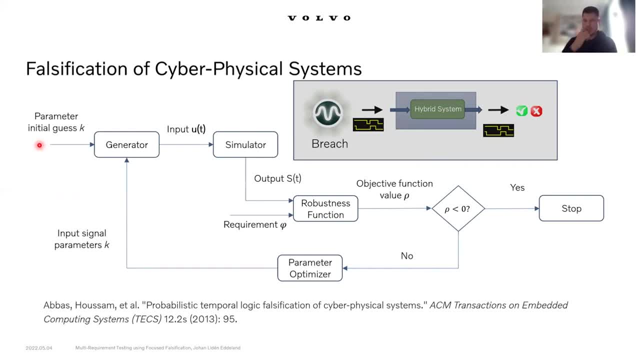 so that we have a set of parameters that will give us the time varying curves that we send into the simulator. So we start off with having an initial guess of these parameters that we send into the input generator to get the actual time varying input signals to the simulator. 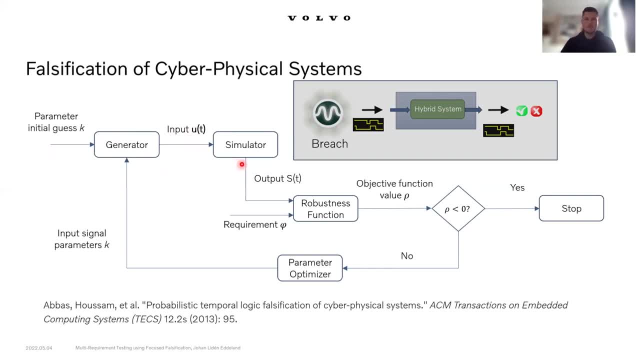 We simulate it, for example using Simulink, and then we get the output. So, together with the requirement phi, which is in signal temporal logic, we can with the robustness function calculate what is then called the robustness value, rho typically, or in our case an objective function value that we optimize over. 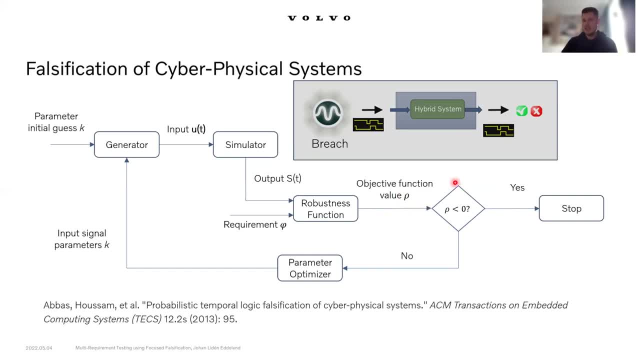 So we check whether this is negative, and if it is negative, then it turns out that we have actually falsified the requirement. So we can stop And we have a counter example that we can give to the developer of the system, If it's not negative. 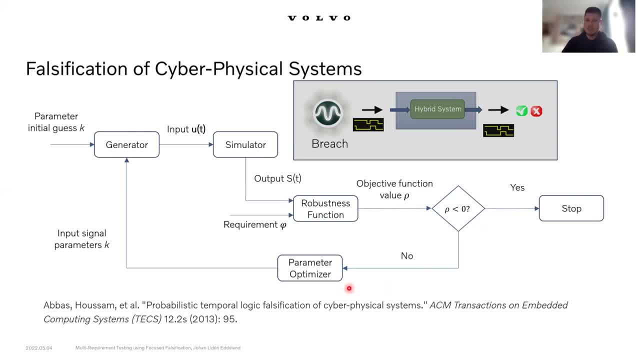 then we take the robustness value and we send it to a general optimization solver in order to find new input signal parameters where the goal of this optimization problem is to minimize this rho the robustness value, Because, as I said, if it's negative, then we have found a counter example and that's what we're after. 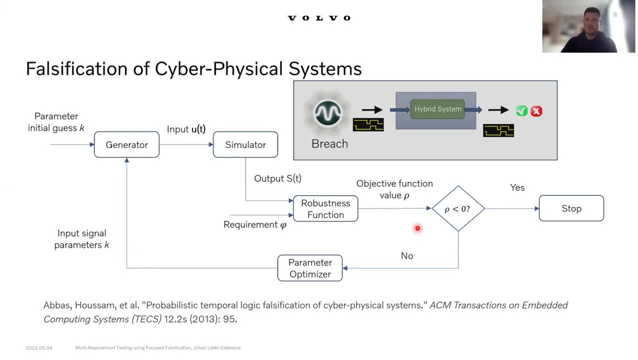 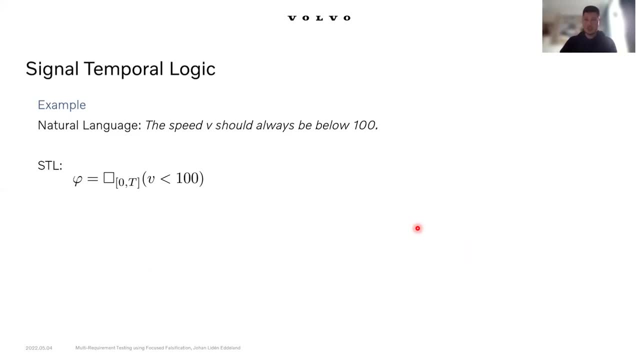 Now this is made possible by signal temporal logic and the way signal temporal logic specifications work. So I will briefly show this with a simple example. So we'll assume here that we have the natural language specification that the speed v should always be below 100.. 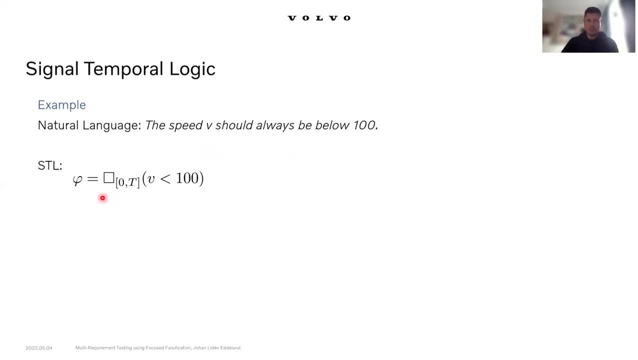 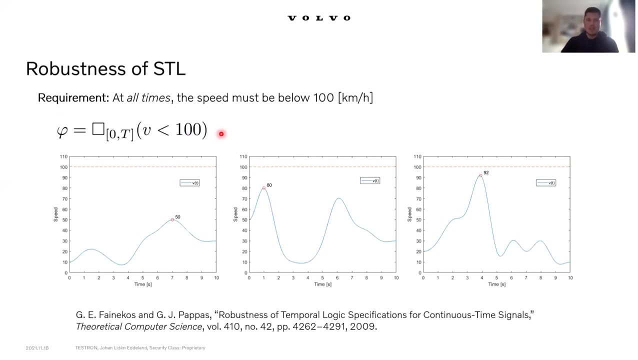 The corresponding STL specification looks like this: That we have this box operator, which means always in this time interval, and then we have a predicate which has v less than 100.. Right So now, assuming that we have this specification and we have these three simulations, 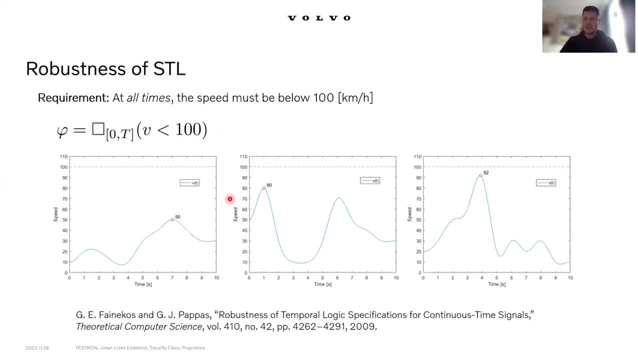 where I have plotted v as a function of time in all three of them. if I ask the question which one of these is closest to falsifying the requirement which says that we should be below this dashed line 100 kilometers an hour, then I think many of us would say that the right one is the closest. 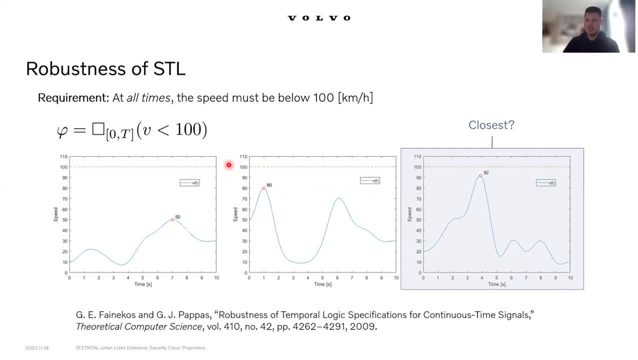 simply because the maximum value of the speed over the entire simulation is closest to the threshold. Now, for this specific example, this is exactly how the robustness is calculated. It's simply the difference between the threshold value to the maximum of the speed with the entire simulation. 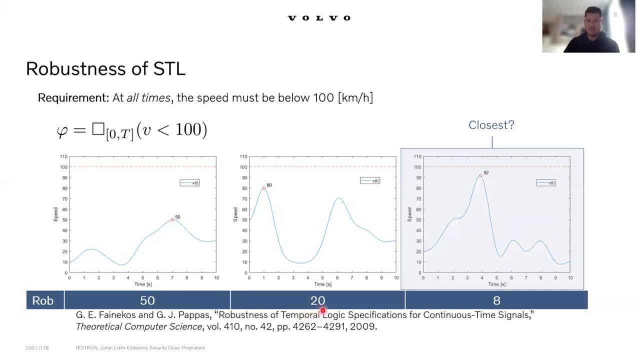 So the robustness value for the left one would be 50, for the middle one 20 and for the right one it would be 8.. But the good thing about robustness of STL specifications, STL requirements, is that it can be calculated for any STL formulas. 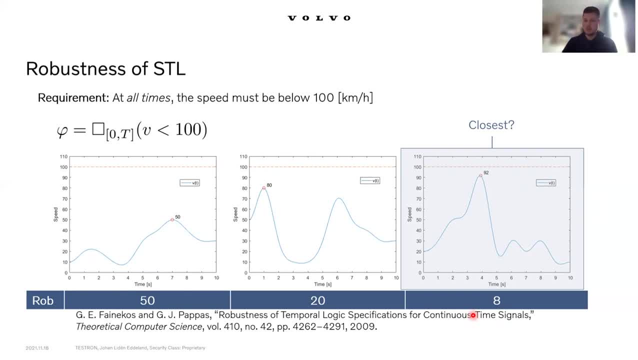 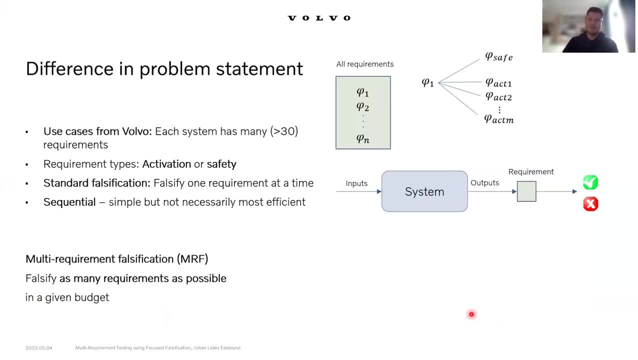 So, which makes it very good when we want to use it in a falsification framework. Now, there is a difference, however, in the problem that we want to solve, based on the use cases we have from Volvo, compared to the standard falsification procedure which I just presented. 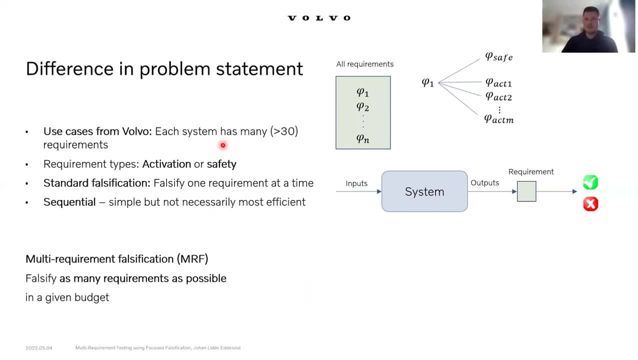 So in the use cases from Volvo, we typically have many requirements for each system, more than 30, let's say. We also have different requirement types. So each requirement- let's say phi1- we can see over here- it has one safety component which must always be fulfilled. 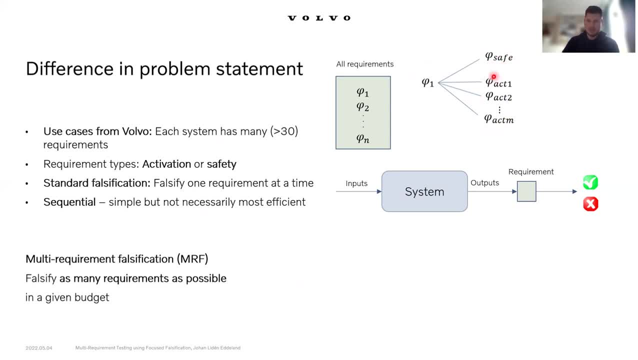 and it has zero or more activation components, which and each one of these says when you have activated a part of the requirement, so it's used for a different purpose than the safety one, which we'll come to later as well. But the important part here is that 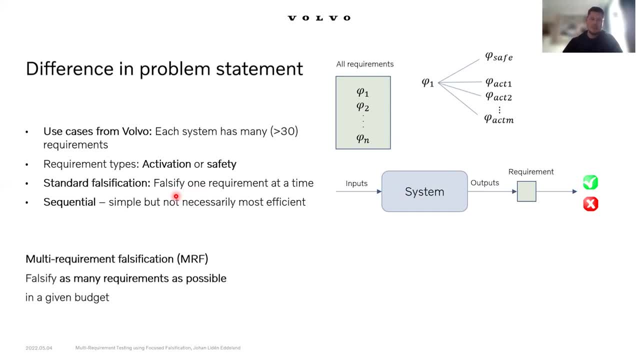 the standard falsification procedure. it really only takes into account that you falsify one requirement at a time. But, for example, if we have a lot of requirements, so in what order should we do that? The most naive implementation of this, or the simple one, would be to do it sequentially, right? 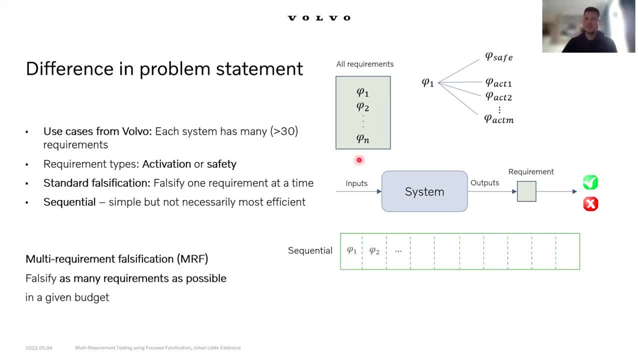 You choose some kind of order, maybe arbitrarily. you order your requirements and then you spend some simulations for each, trying to falsify them. So it would look like we have this box of requirements. first we take the first one, based on some ordering, then we take the second one. 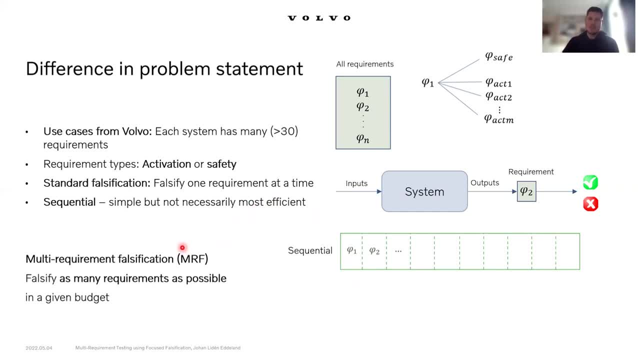 and so forth until we reach the end. What we propose here, we call MRF- Multi-Requirement Falsification- where the problem is to falsify as many requirements as possible in a given budget. So we present here an algorithm with three different phases that attempts to solve this problem. 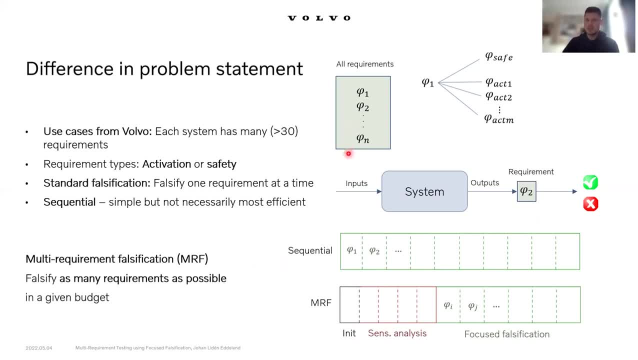 in a more elegant way. So, in short, what we do is that we take this entire box of requirements and try to consider them all at once when we falsify them, instead of just sequentially. So now I will spend the next few seconds going through the different phases. 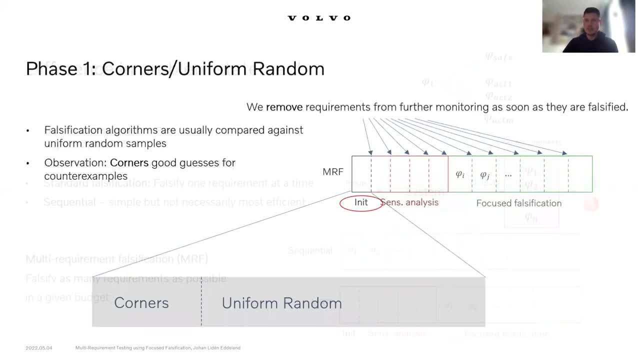 of this algorithm that we are proposing here in this paper, the MRF algorithm. Now the first phase, which I call INIT, here is corners and uniform random sampling, where we can see that typically falsification algorithms are compared against uniform random samples in the parameter space. 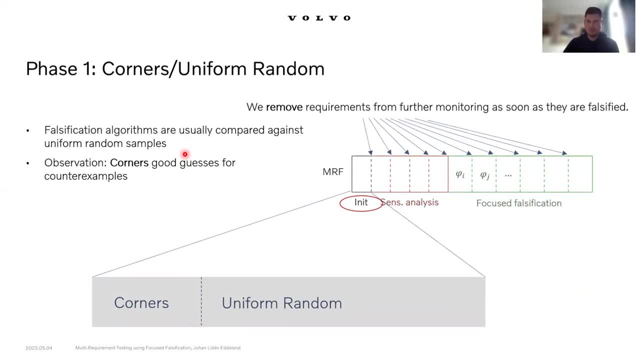 But we have observed from previous public benchmarks that corners are good guesses for counter-examples, so we should include them as well in an initial phase, And corners here. a corner is when the parameters have either their minimum or their maximum value from their allowed range, which intuitively is a corner. 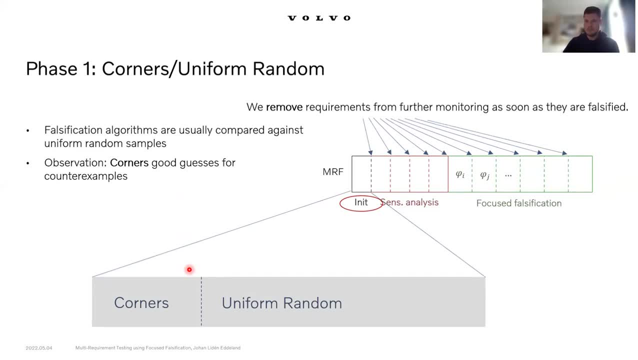 if you plot them in the parameter space And then. so first some corner samples and then some uniform random samples, And we can also note here that at regular intervals we remove requirements from further monitoring as soon as they are falsified. so the list of requirements. 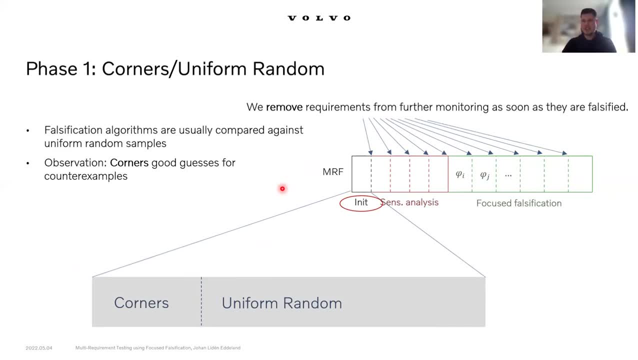 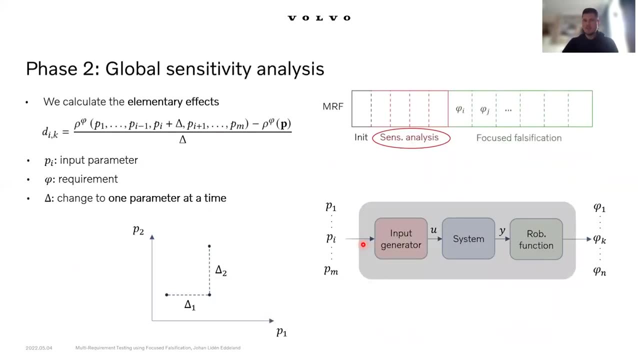 that we are considering for falsification. it shrinks over time the more of them we falsify. Then, when we have done this initial step, we do the global sensitivity analysis. this is the global sensitivity analysis, where we calculate the elementary effects of each input parameter. 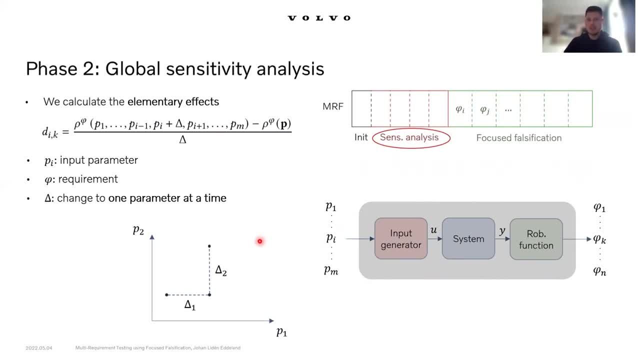 So what we do is that we change one parameter at a time to create a path in the parameter space, to then see which parameter affects which requirements by the use of the robustness values. So as an example here in two dimensions, we start from an initial random point. 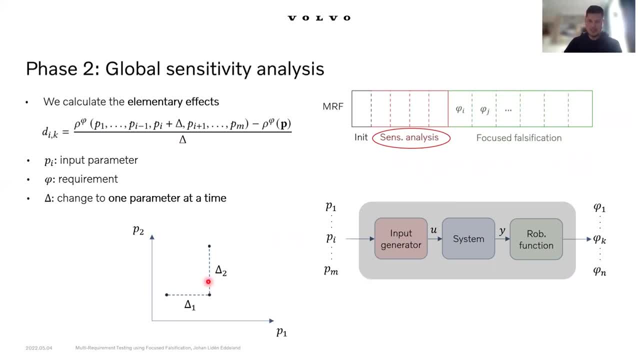 then we take a step in only parameter one, and then a step in only parameter two, And then, if we have more, we take a step in only parameter three, and so forth. So by repeating several such paths, we get an approximation of which parameters affect which robustness values. 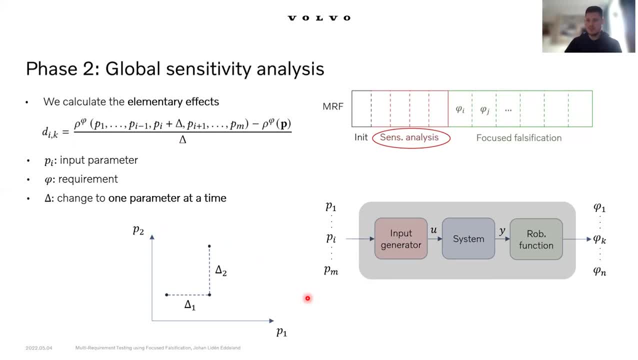 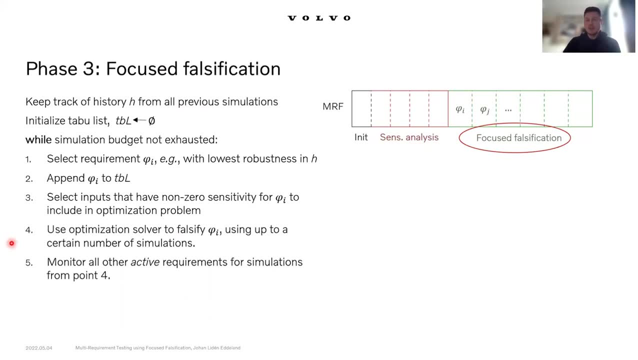 And this is something that we use in the next phase, which is called focused falsification. So I present this phase as a pseudocode kind of an algorithm here where, in short, we keep track of the history from all previous simulations, from the initial phase, sensitivity analysis. 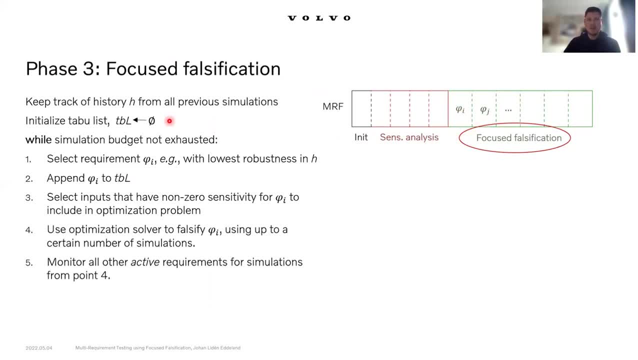 and previous iterations of the focused falsification. We have a taboo list which we initialize to the empty set, which we simply have there to make sure that we don't focus one requirement several times before all other ones have been focused already. So then we loop. 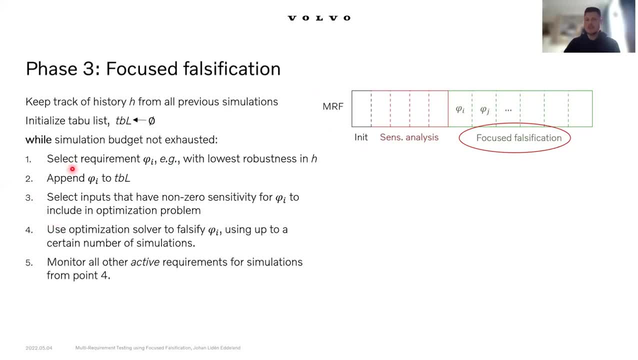 these five steps here. The first one is that we select requirement based on some heuristic: for example, the one with lowest robustness so far, We append it to the taboo list so we don't repeat it more times, as I mentioned. And then we select inputs. 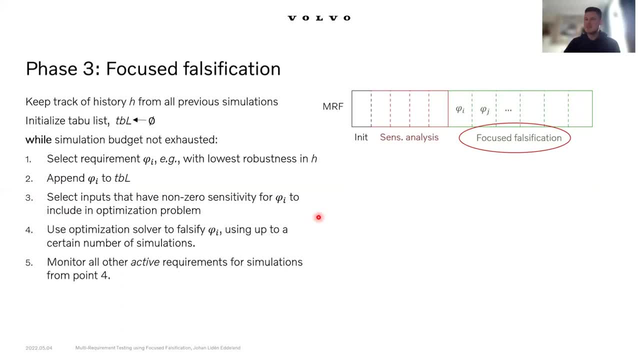 that have non-zero sensitivity for the specific requirement. So this is where we use the sensitivity analysis results. So those are the only ones that we include in the optimization problem. So step three here is used to reduce the dimensionality of the optimization problem. 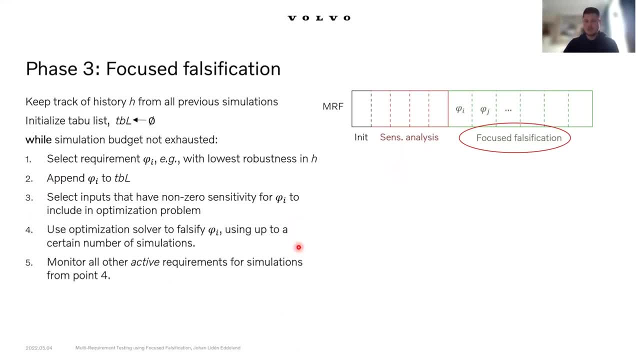 And then number four is essentially the standard falsification procedure. We use an optimization solver to falsify the requirement. And then number five: we store all of these simulations in step number four and we monitor all other active requirements that we still have in our active list. 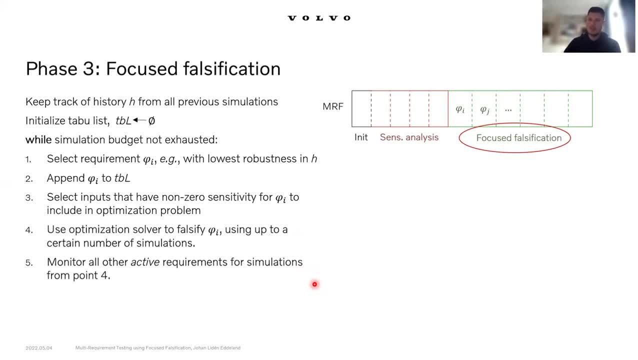 to make sure that, for every simulation that we have, during all of these steps, we always monitor all requirements, because we need to access their history as well, And a note here is that, while we only include parameters that are non-zero sensitivity in the optimization problem, we still vary. 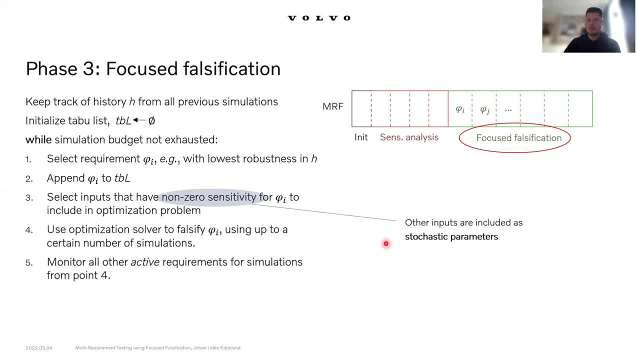 the other ones. so we call them stochastic parameters because they are varied randomly and the optimization solver is not aware of them, But it's still important for us to vary them, since other requirements are still active that might be sensitive to other parameters than the current requirements. 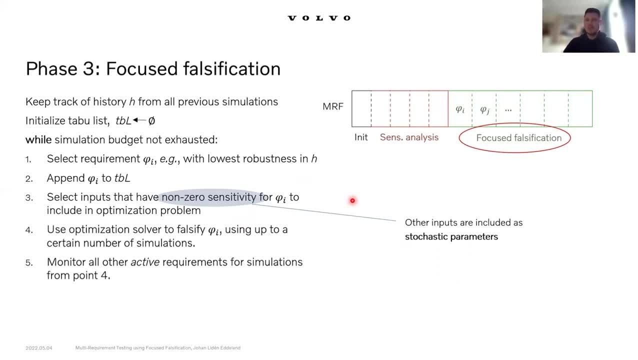 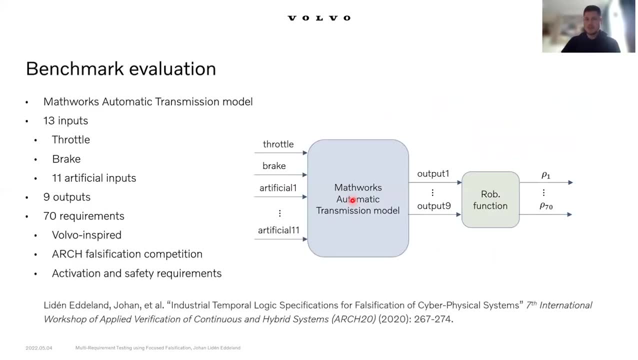 being focused. So that finishes the discussion on this proposed algorithm that we have. So what we have done, then, is that we have evaluated it on a benchmark, and this benchmark is an extension of the MathWorks automatic transmission model, where we have 13 inputs, the standard throttle and brake. 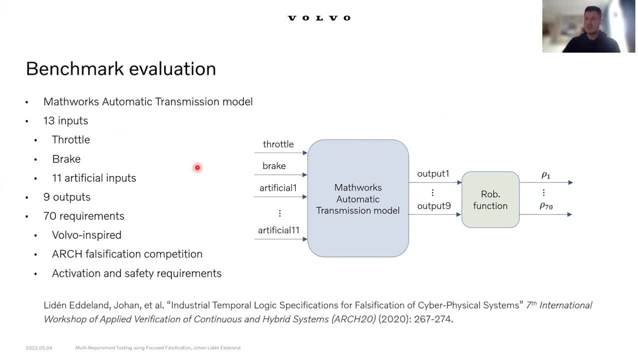 and then 11 artificial inputs which affect the requirements but they don't affect the dynamics of the model. Thank you. We have nine outputs in total and in total there are 70 requirements, where most of them are inspired from Volvo specifications, Volvo requirements, and they are published. 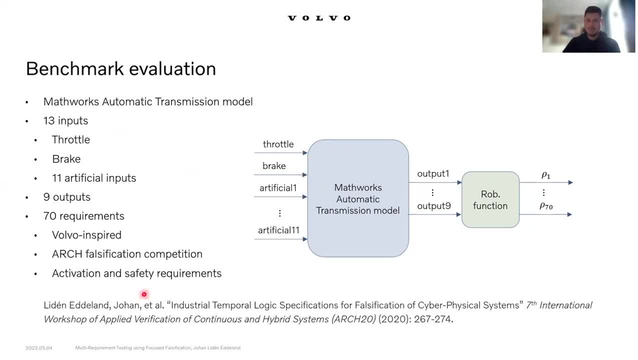 in a separate works, a benchmark publication, and then some of them are the requirements from the ARCH yearly competition on falsification, and we should note that all the requirements have activation and safety components as well. So there are some of the requirements that we have that we have. 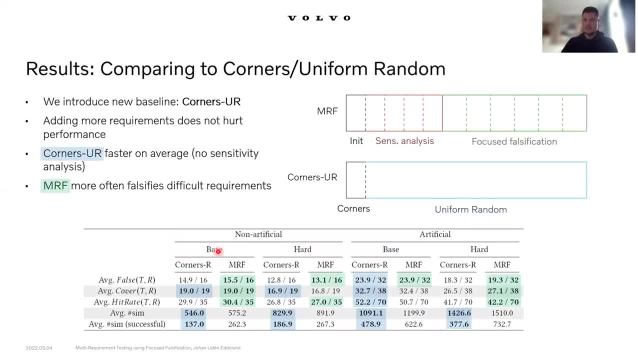 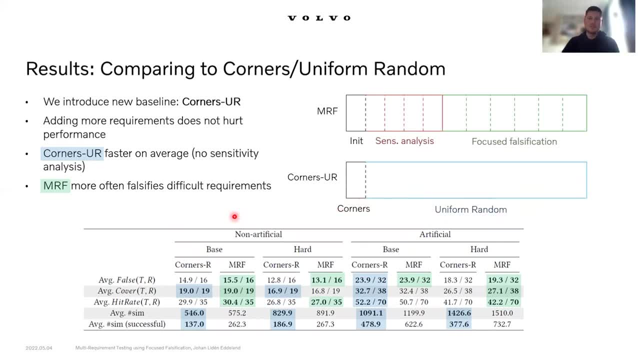 and then the rest. we do uniform random samples and this performs very well as a baseline because adding more requirements does not hurt the performance, unlike MRF where more requirements, it's difficult to fit them into the simulation that we have, of course. so the results are presented. 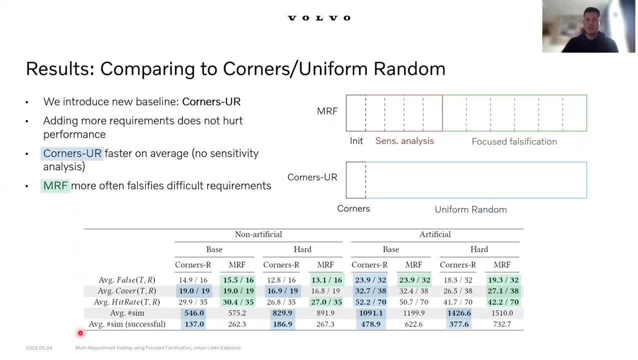 here in this table, which is also shown, but without colors in the paper. I have color coded it now, with blue for whenever the baseline is better and green when MRF is better. so what we can see from these results is that corners, uniform, random is faster on average.